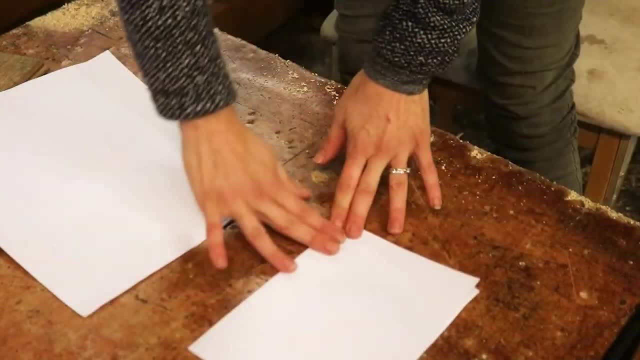 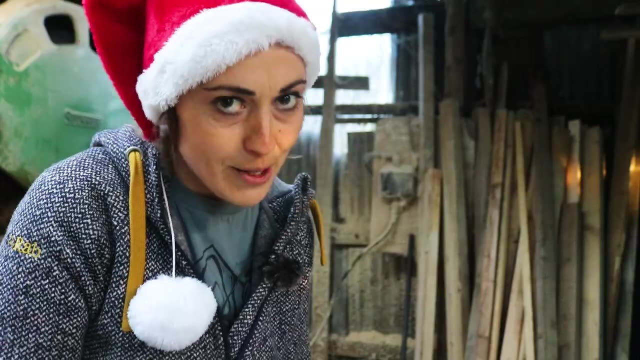 even consider buying a template, because all you need to do is fold a piece of paper in half, cut out a shape, draw around it on an off-cut piece of hardwood, drill your thumb hole, cut it out. A lot of people told me as well that they swear by them when they've got arthritis in. 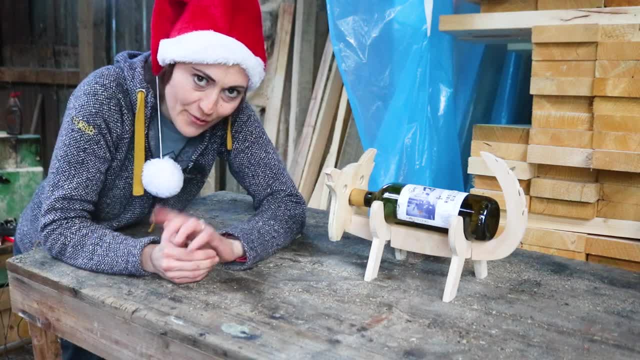 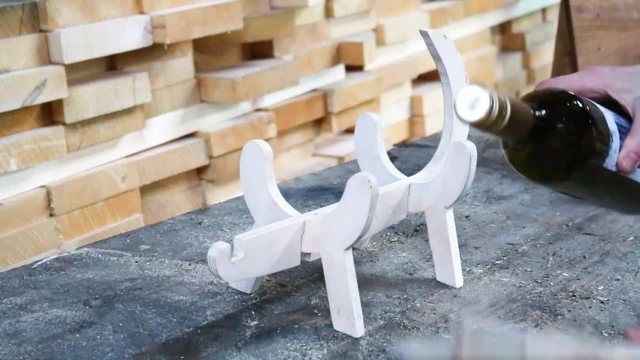 their hands and it's easy to hold the book open. Number three is perfect for anyone like me who likes a glass of wine And dogs. This is one of my absolute favourites out of all of them because I enjoyed designing it. I started drawing on folded paper, which a lot of these projects were done. 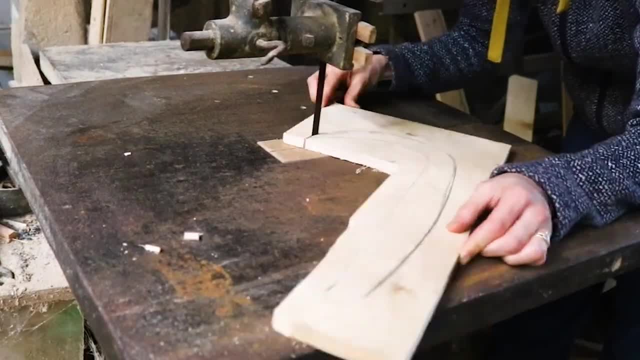 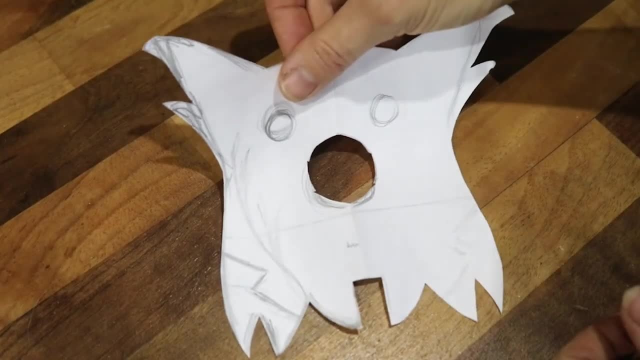 and cut everything out on a bandsaw and just used a scrap piece of plywood as well. The other thing I really like is, if this doesn't look like your dog, you can easily change the tail, the face or create it as a different animal. And while I was making it, 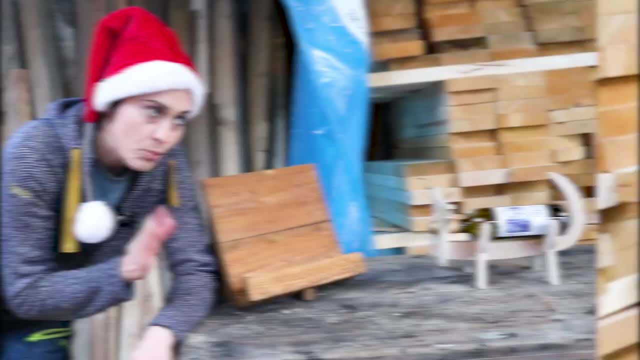 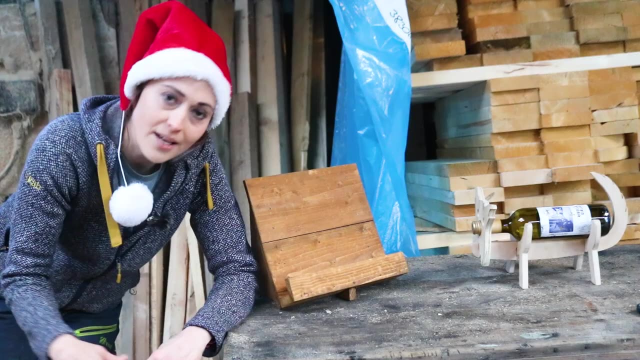 it even looked like an alligator or crocodile. We've all got to eat, so there's no surprise that you're bound to know a foodie lover in your life. This cookbook stand is a doddle to make. Okay, I didn't bring a cookbook today. 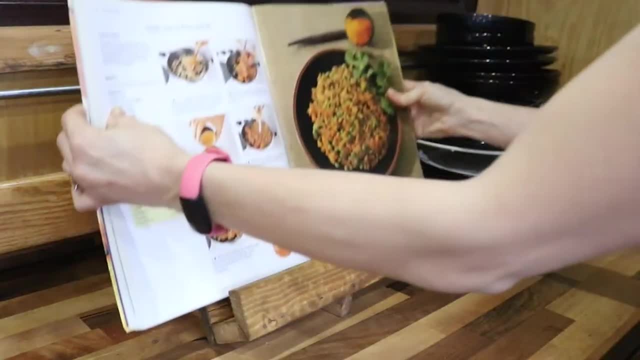 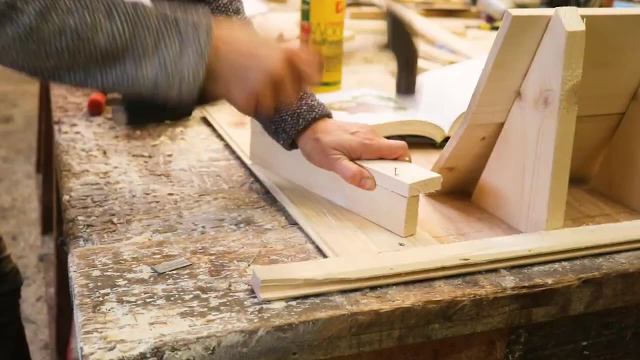 but all you have to do is place the book there. This is all made from scrap pieces I found lying around. but you don't even have to have it in panels. You could have a solid piece there. you could change the dimensions of this lip and even paint it to match the person's kitchen. 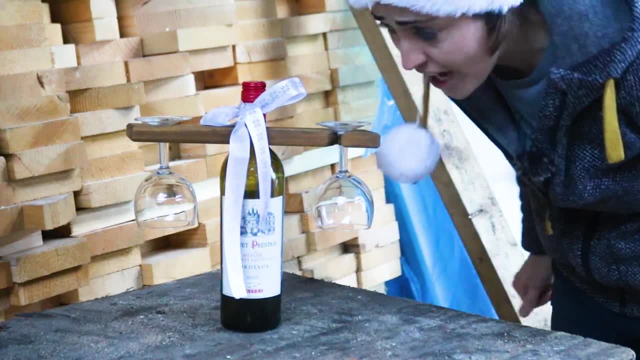 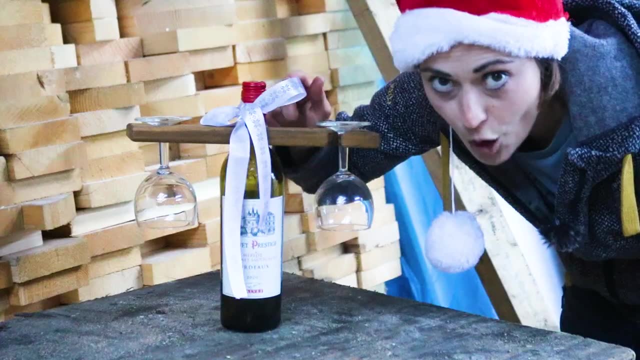 Number five actually started out as a component from a really old chair, and now I think it's quite fancy because it's presenting a bottle of wine and two glasses to form a caddy. Don't forget that. But all it is is a piece of wood with a drilled hole in the center. Let's just take that. 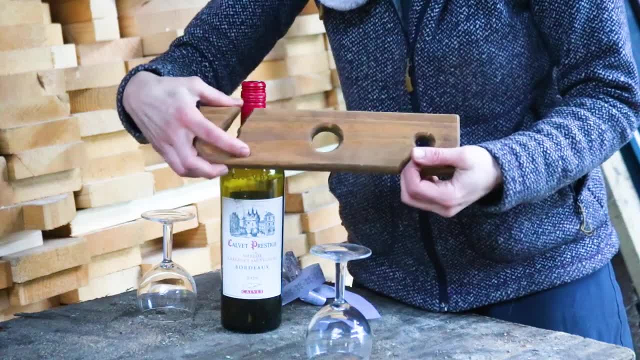 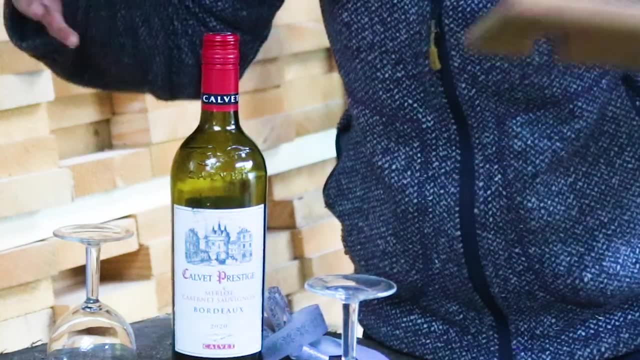 bow off And another two holes either side for the glasses and some notches cut out. It doesn't even have to be hardwood, You could stain it, varnish it and just present that as somebody. It just pimps up a cheap-ish bottle of wine. Now, a lot of you told me number six was your favorite. 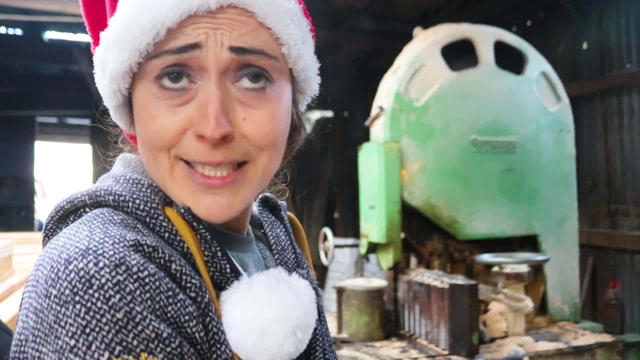 which kind of hurt, because it was my husband's idea and I told him what a ridiculously saucy thing to make. And then the next day I thought that's genius- A cat bum bottle. I thought that's genius. I thought that's genius. I thought that's genius- A cat bum. 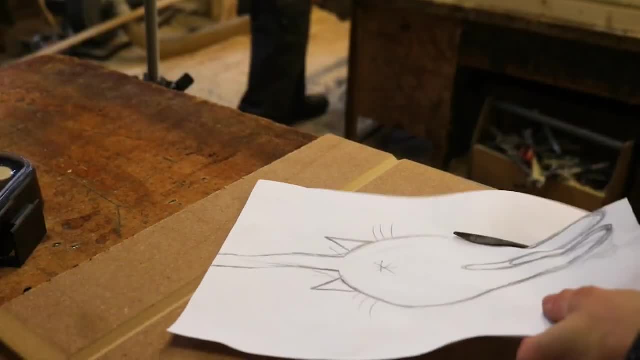 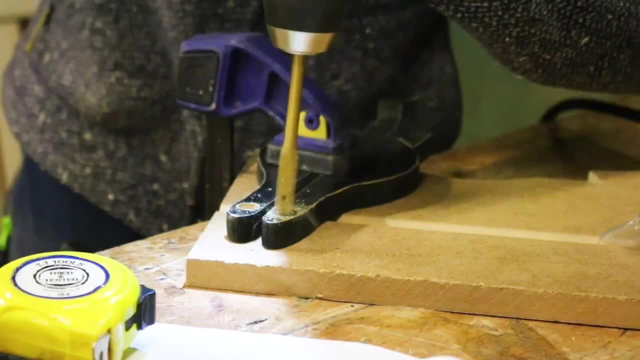 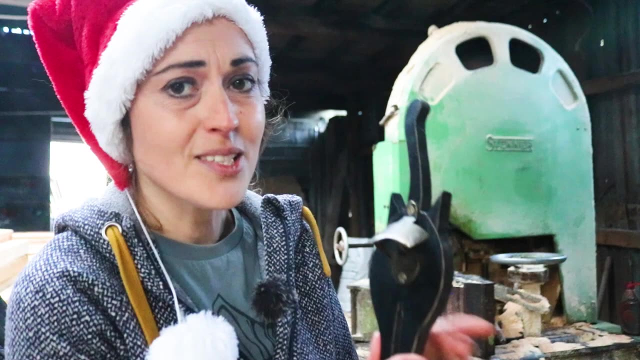 cut it out of MDF, drilled some holes in the pores for magnets, added a bottle opener, screwed it to a wall. Oh, and I did add some whiskers for effect. This is going to be sent to a friend anytime soon who has a cat, But you could personalize it with a black and white cat. 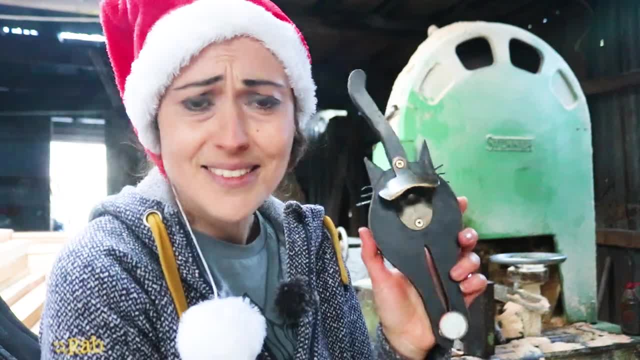 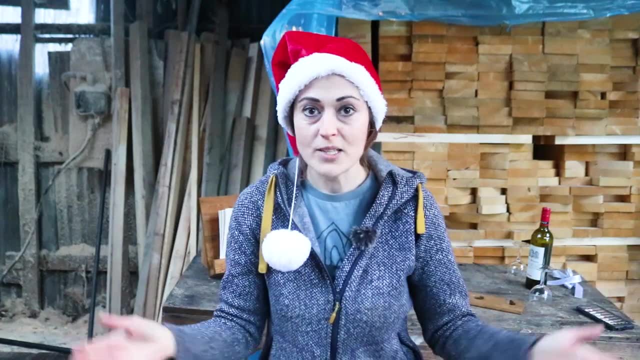 or whatever you like. You know what I want: to make: more of these. I think they're just so much fun. For number seven, I've got to go back to some footage because I've given them away, But I showed you how to make some really. 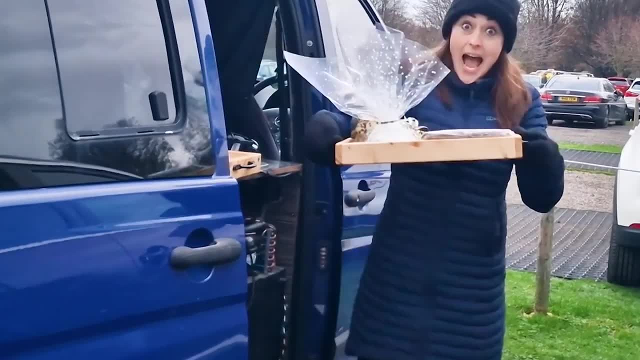 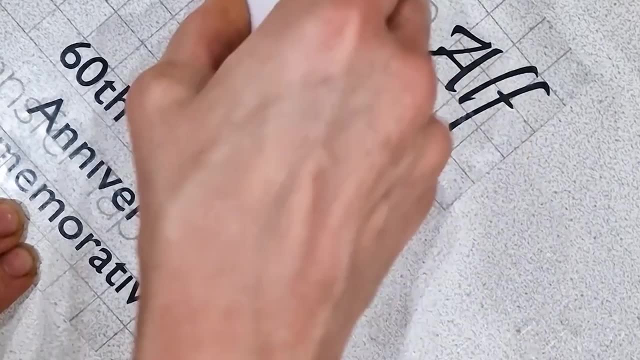 basic food trays, some serving trays, And that was to treat them as bases for gift hampers where I would fill them with other goodies, put handles on the sides and personalize the bottom. You could create a Santa tray or anything you want. I did mine with a vinyl cutter And when you've 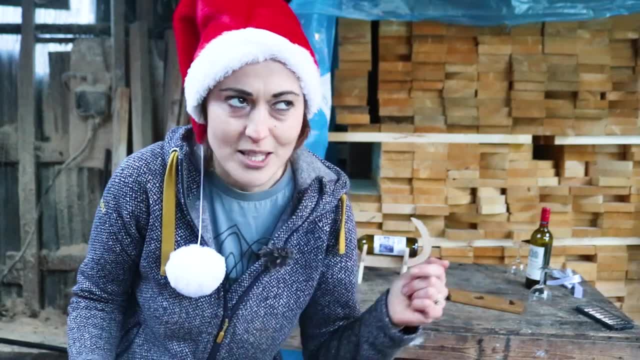 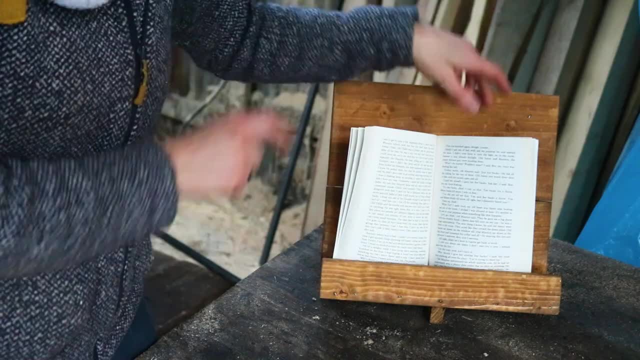 got loads of family members to buy things for, you start questioning whether to pay six to ten pounds for a wicker basket. So those actually saved me a fortune. For number eight, we're going to go back to gifts for book lovers, And this is actually one of the cheapest gifts that I've ever. 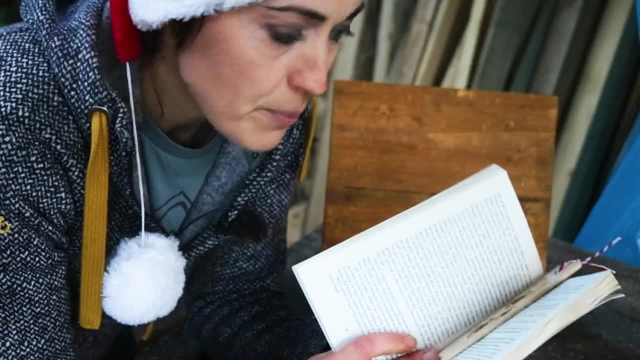 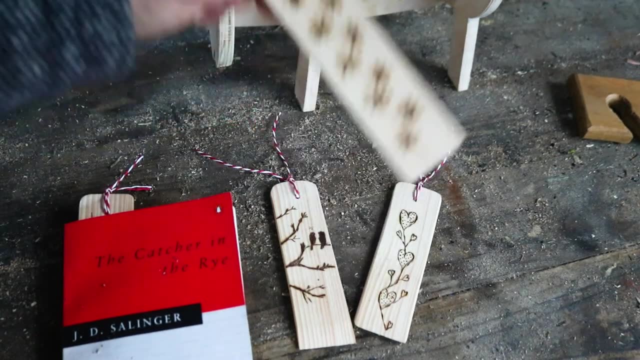 seen. It's one of the cheapest gifts you can make out of all of these, And they're really easy to make. personalized bookmarks made out of wood. Not only did I love how cheap they were to make as stocking fillers, the thing I love the most is that you can personalize them for somebody who 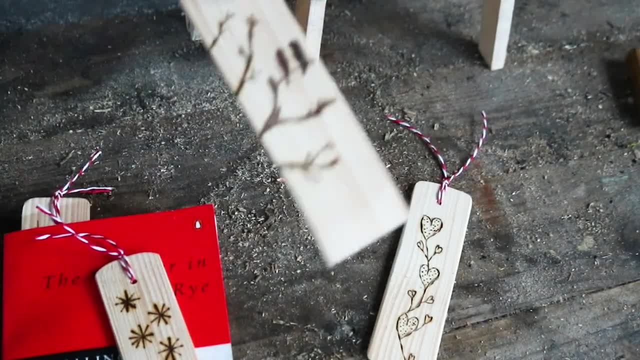 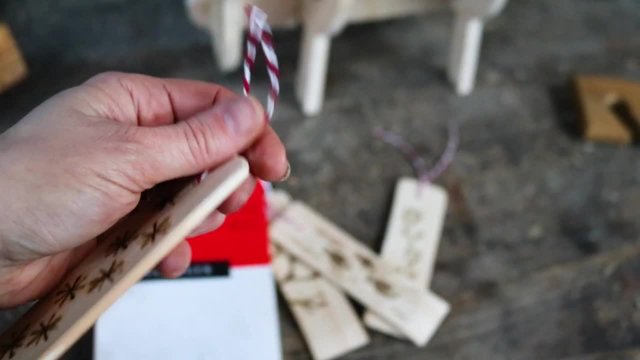 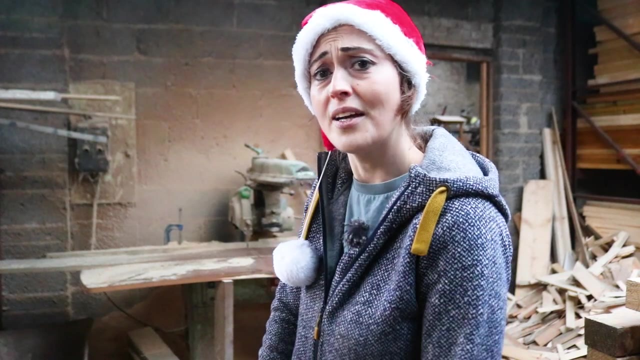 loves other hobbies, like flowers, nature, fishing And just draw whatever you want first and then just go over it with a pyrography pen. And I just use cheap fancy ribbons, Number nine. you might start to think I've got a drinking problem by now, but I know a lot of people who do like a tipple. 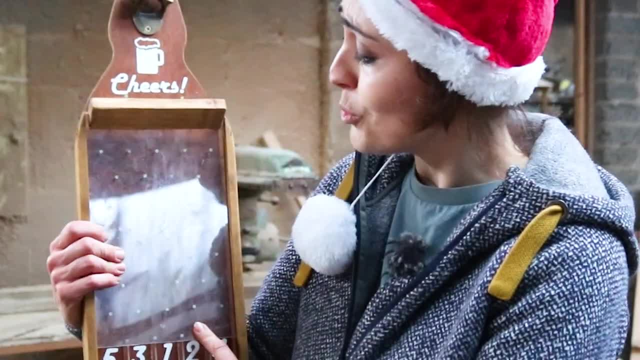 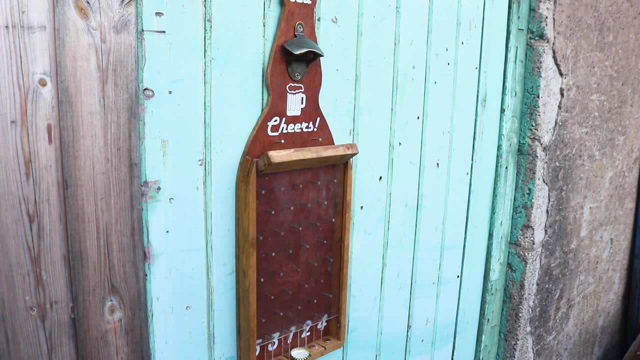 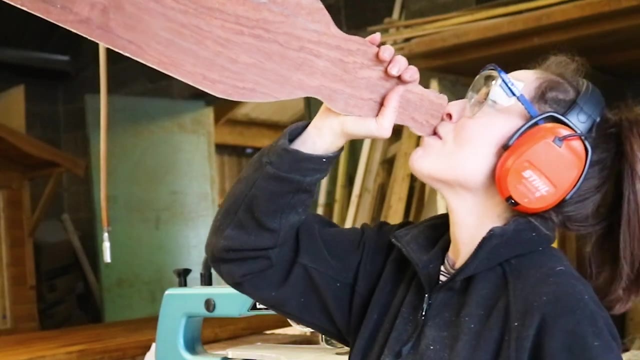 and that is a Drinko Plinko game board bottle opener. This actually took me quite a bit of tinkering to sort out because there's a few moving parts, but it was by far one of the most enjoyable to make. I've drawn out the beer template for you to download And after cutting that out, 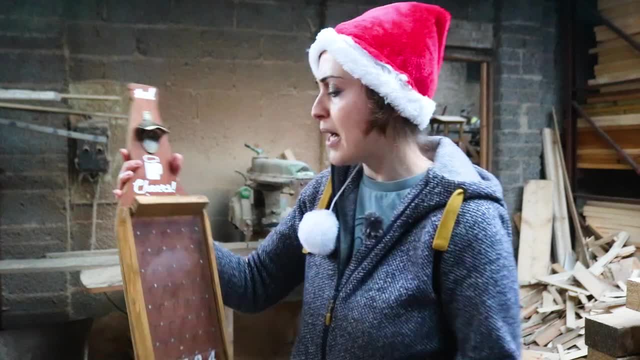 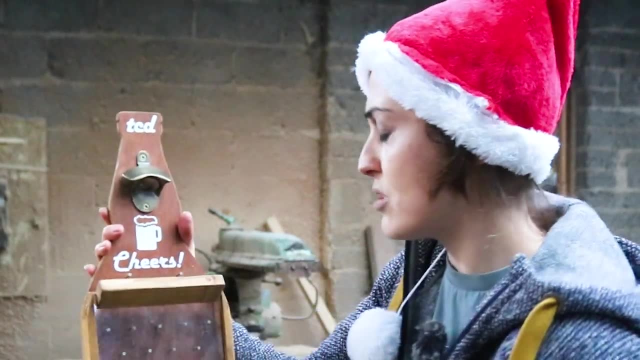 I just hammered in a load of nails which have to be in a certain sequence. Mine are one and a quarter inch apart. You could get away with one and a half, but no less than one and a quarter. things will get stuck and they've got to be zigzagged. Believe it or not, these were all from. 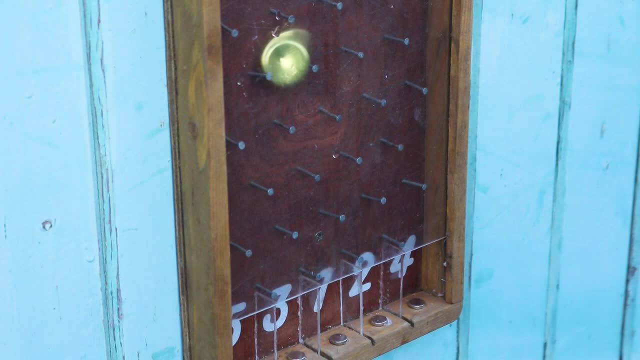 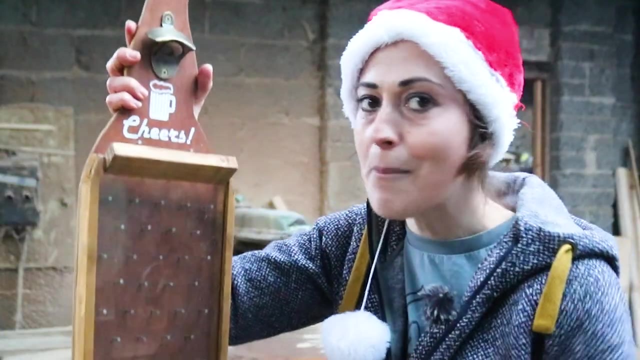 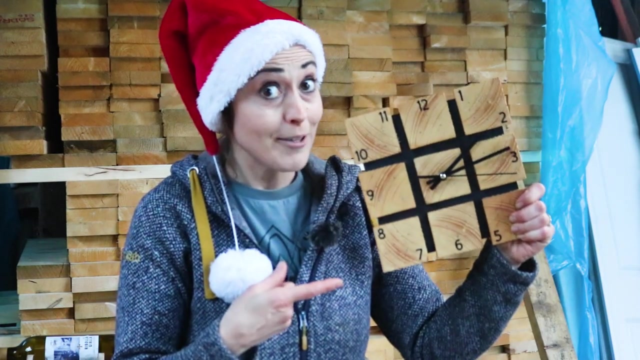 offcuts, And when you open a beer it just staggers its way down. I love the clinking noise. And then right in the bottom there's a scoring system and some magnets. I think this is perfect for a man cave, woman cave. just love it. It's about time you made number 10.. It's an offcut clock. This was. 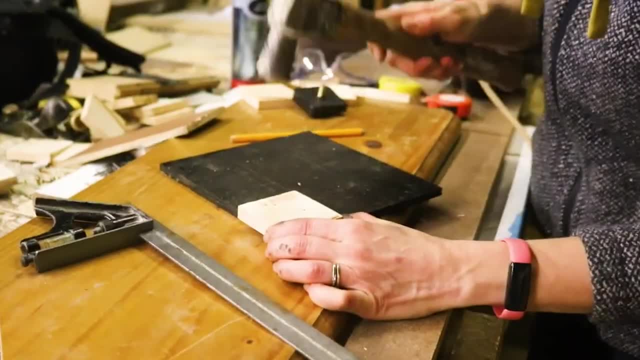 so cheap to make, because all I did was cut up an old fence post, cut it into slices- clattered a piece of wood at the back, and then I cut it into slices. and then I cut it into pieces of wood at the back and then I cut it into slices. clattered a piece of wood at the back, and then I cut it into. 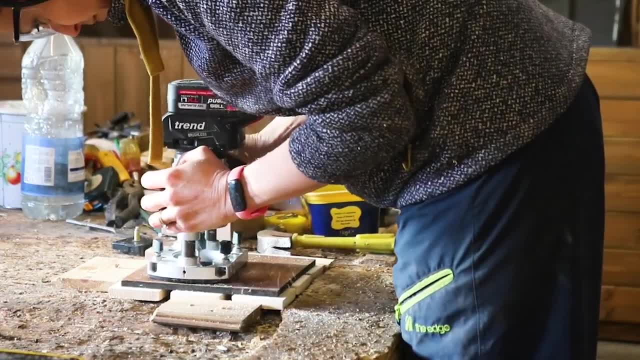 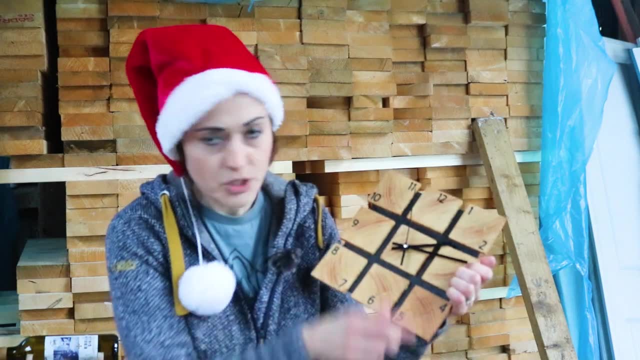 pieces of wood at the back and then I cut it into pieces of wood at the back and then I routed a hole for the clock to go through. Then, if you wanted, you can personalize with numbers, but you don't have to use squares. You could add slices from a tree trunk, You could paint it, do whatever you. 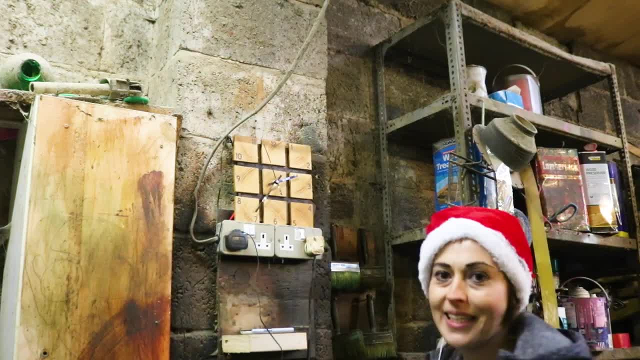 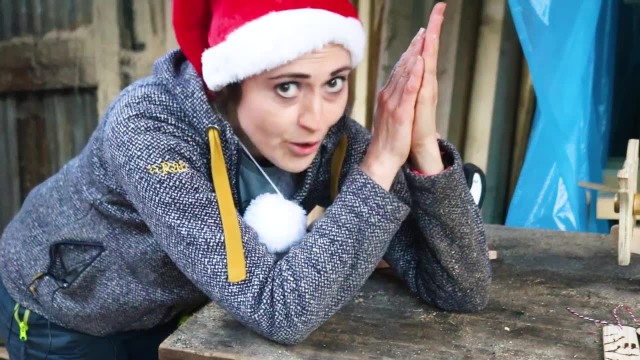 want. I just think this would be great in a dad's workshop, a mum's craft room or vice versa. You get the gist For number 11,. this has to be one of my absolute favorites And it's ideal for anyone. 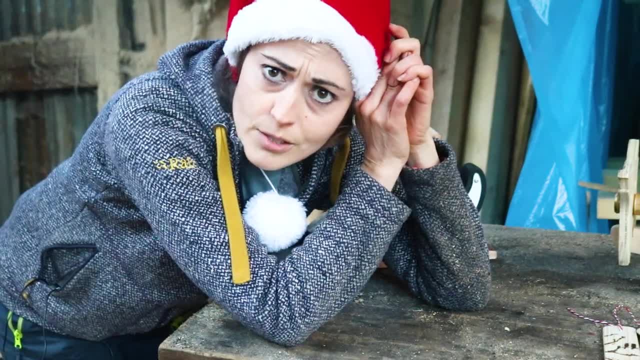 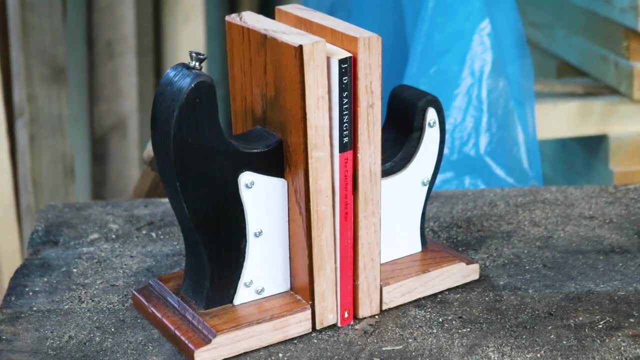 who loves to play guitar or loves to listen to rock and roll. I'm going to go with number 11.. It's my guitar bookends. Let me know in the comments if you genuinely think this looks like a cut-up Fender guitar And it was actually one of the quickest projects out of all of these to 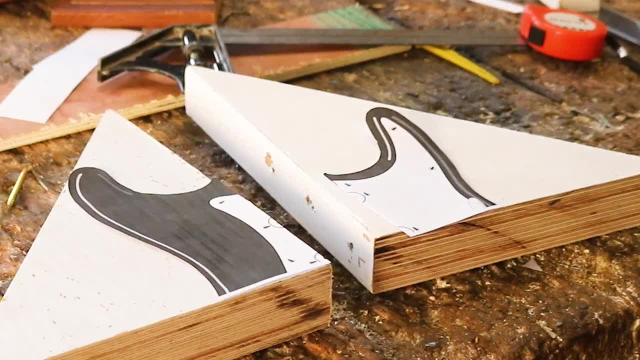 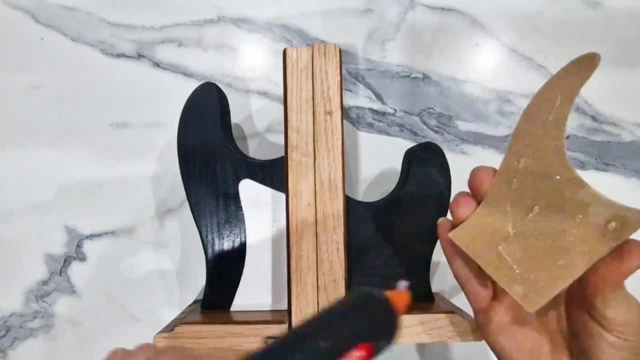 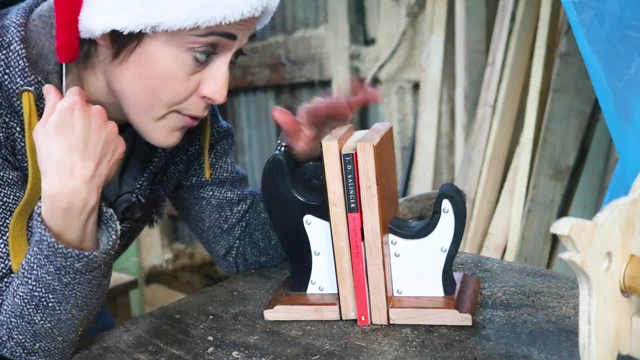 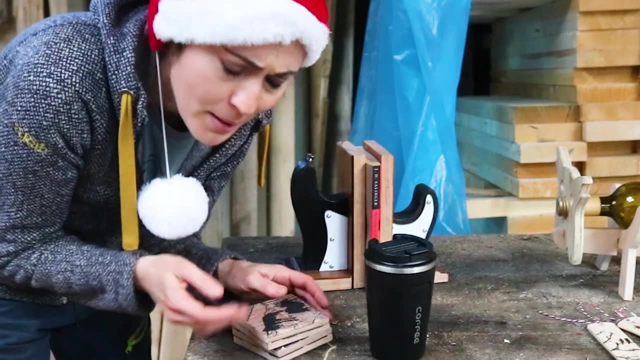 this is cool And I can't wait to give this to my brother for Christmas. Number 12 is for anyone who likes a cuppa- And most of us do, don't we? I've always got to have a coffee near me. This is just Sapele off-cuts, but you don't have to do this with hardwood. 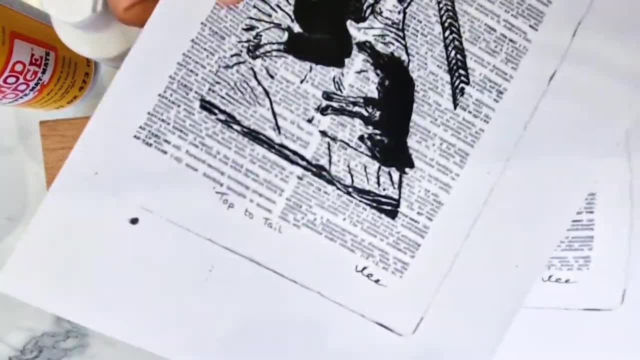 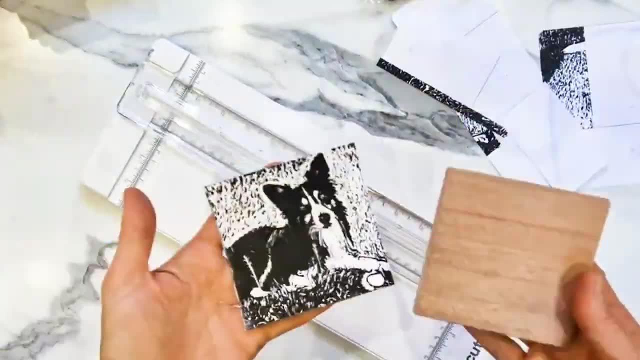 You could do this with softwood as well, And what I did was go to my local library, had some prints done, but there were LaserJet photocopies for my original Linocut prints. I used some Mod Podge to transfer the images straight to the coasters.